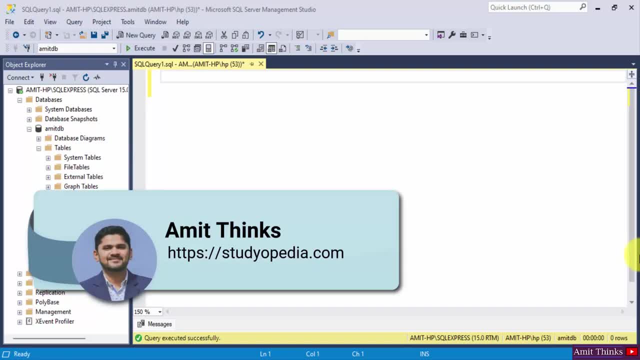 Hello guys, welcome to Amit thinks. In this video we will see how we can work with SQL: create view statement to create a view. So what is a view? A view in SQL is basically a virtual table which is based on the result set of an SQL statement. So if you want to show or present a specific data from your database or table, you can use a view. A view basically contains rows and columns. that is part of your records. Okay, the fields in a view are basically fields from one of your tables. 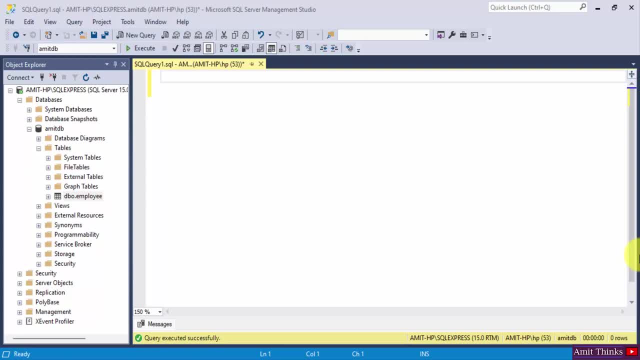 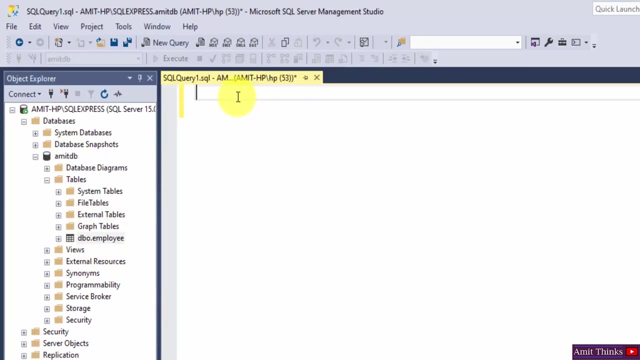 Only, as I told you before, so you can present a data in a more readable form using view. So to create a view, we use the create view statement in SQL. So let us see an example here in we have Amit DB database you can see, and an employee table. Let us enter the database using the use command. use space, database name. that is Amit DB is our database here. Execute and you can see successful. Now let us enter. 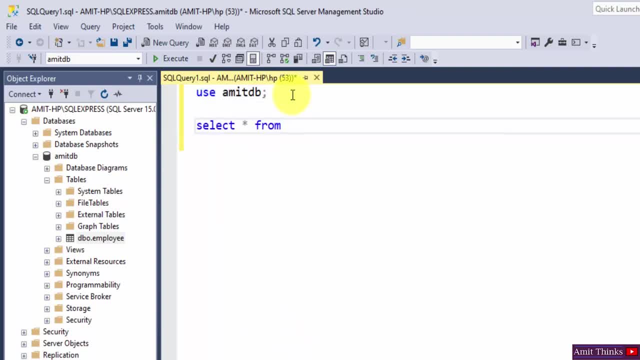 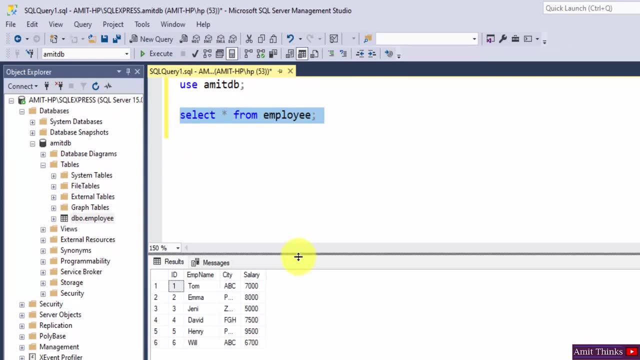 our table. Now let us see the records of our table. Select star from employee, select it and click on execute. Now here and you can see our record is having ID, employee ID, employee name, employee city and employee salary. Now let's say we need to create a view for employees with city ABC, that is, the employees that is, employees living in city ABC. So that would be the first one and the last one, or we can fetch a view for it. Let us 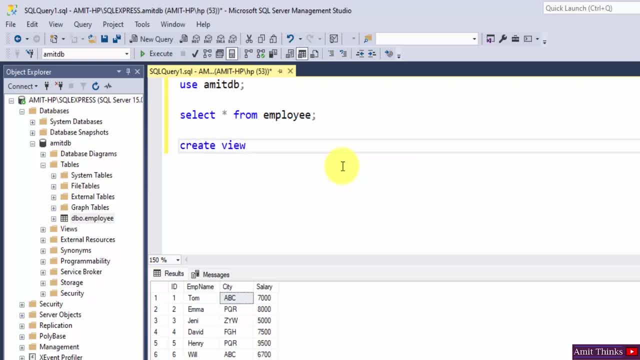 create a view. Create views the command. Let us add the name of our view, Let's say employees, ABC. we can write: use the alias as now, use the select command. So we wanted employee name and city, so EMP name and city from mention the table name. that is our employee. 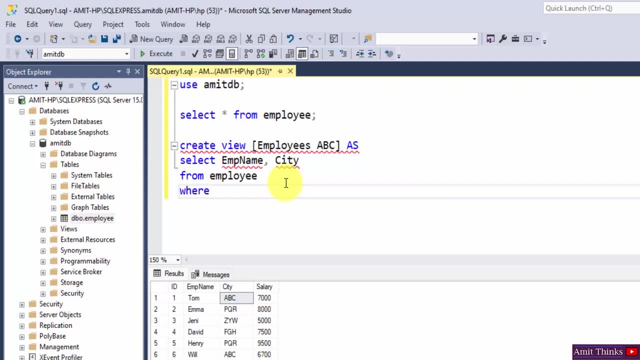 Okay, where city is ABC? Okay, now we have created a view. Okay, semicolon selected and click on execute commands completed. Now to display: use the same select star. Okay, in that, in this case we will be using select star from our view name. because you want to get the view, I'll just 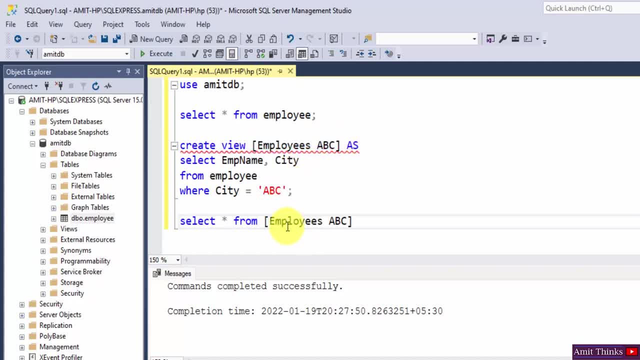 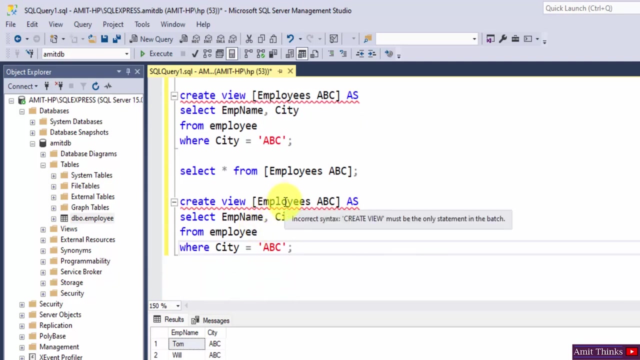 copy this to ease. Okay, so I'll just select a semicolon. I just select, I'll just select and click on execute here and you can see both the records are visible. This is what we wanted for city ABC. Okay, now let's say I'll just copy this again. Let's say we want, let's say we want- to create another view with salary. Let's view the records. 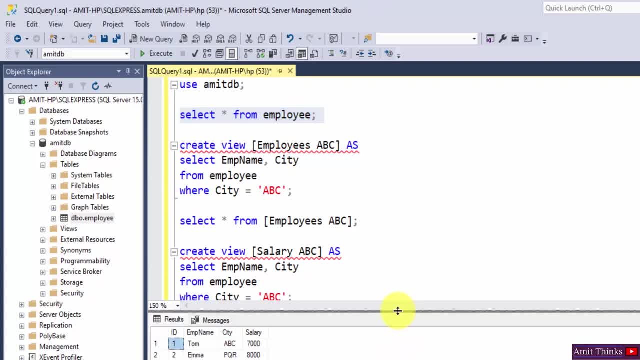 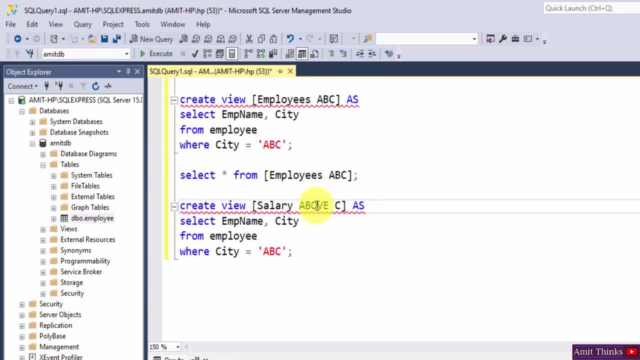 again, select star from employee. let's say we have viewing records with salary greater than 7000. okay, so what we will do, let's write salary above 7000. okay, what we want to display? we want to display, let's say, the employee name and city. let's say: it's fine, we can also display: 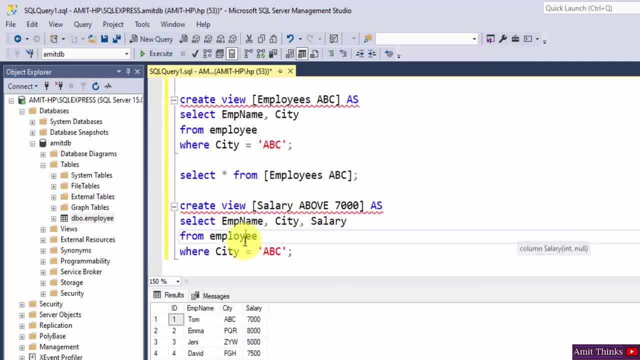 salary also that are above 7000 from employee table wherein. so what condition we need to mention? we need to mention under view wherein salary is greater than 7000. okay, this looks fine, i'll select it. we have a new view now. execute command completed now to display it. i hope you remember it's: select star from. 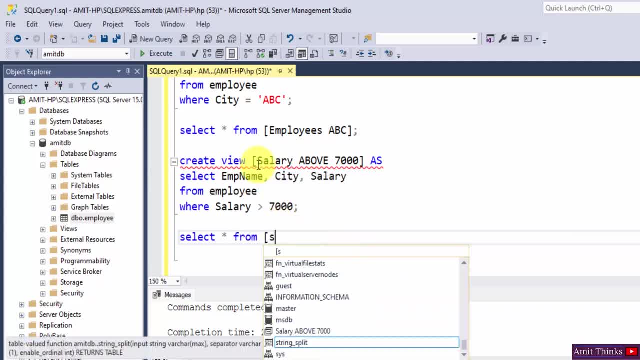 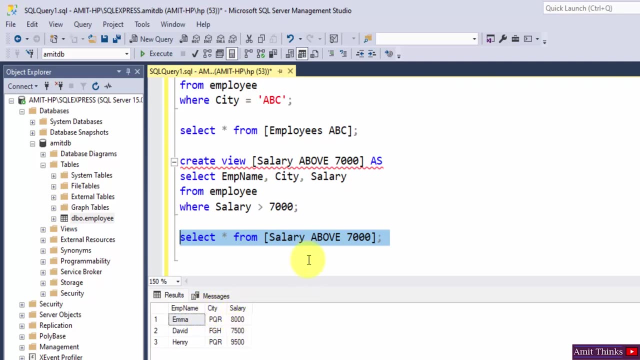 your view name. that is the following- it will come on its own. you can see salary above 7000. that's it. semicolon select and that's it. so we have all the records of employee with salary greater than 7000. okay guys, this is what we displayed using a view. 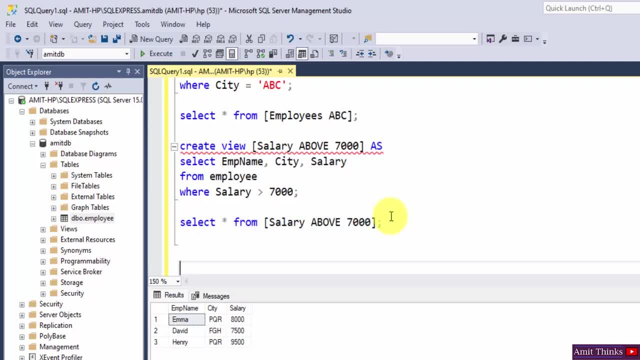 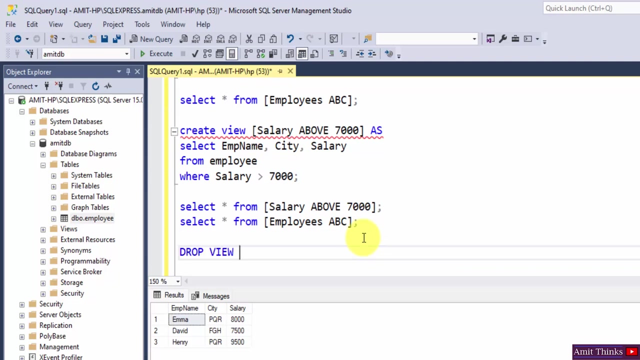 so we created a view now. now we will see how we can remove. so now we have two views here in first, second, both okay. now let's say we need to remove the employees abc view. how we can remove it? for that guys use the drop view command, right drop view and the view name. that's it. so our view name was here it is.